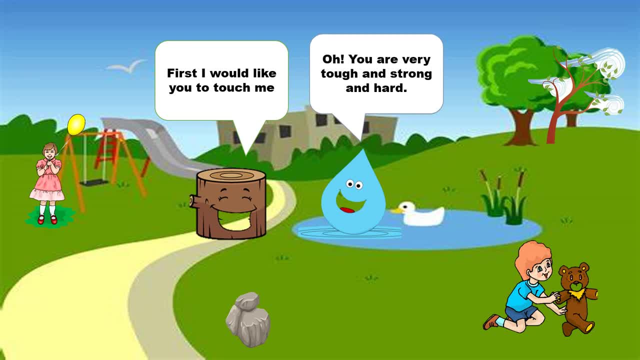 First, I would like you to tell me your name. Oh yeah, You are very tough and strong and hard. Yes, you feel right. That is why people call me solid. Okay, but how you become solid? Because my molecules are very tightly packed and make a proper shape. 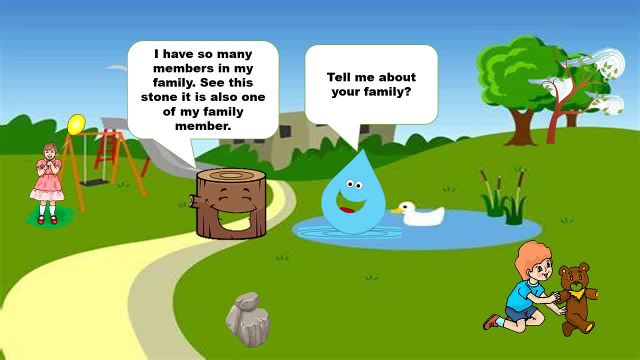 Tell me about your family. I have so many members in my family. See this stone. It is also one of my family members. It means all of your family members are hard, strong and tough. No, no, Some of my family members are soft, light and fluffy. 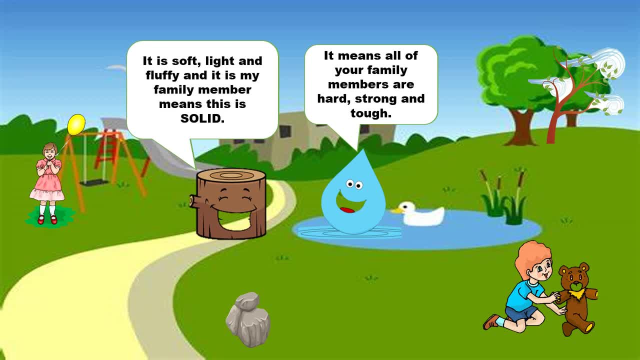 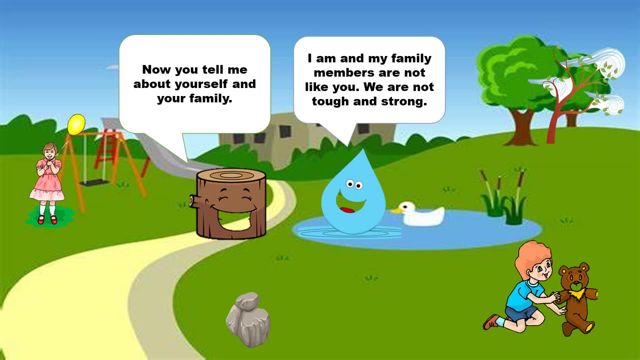 See the teddy bear. The boy is caring, It is soft, light and fluffy And it is my family member Means this is solid, Great. Now you tell me about yourself and your family. I am and my family members are not like you. We are not tough and strong. 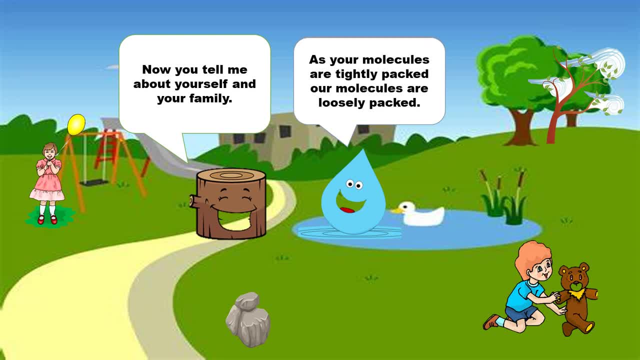 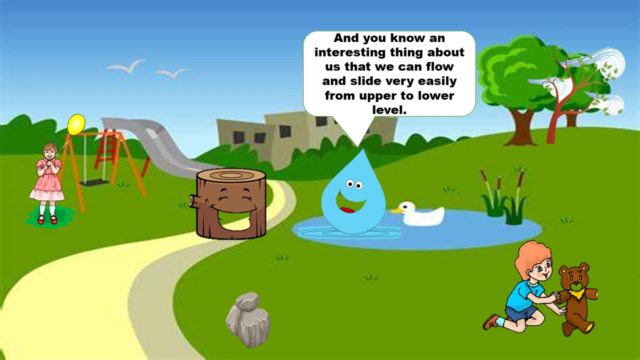 And people call us liquid, As your molecules are tightly packed. our molecules are loosely packed. We have benefit that we can fit in any of the container And you know an interesting thing about us: that we can flow and slide very easily from upper to lower level. 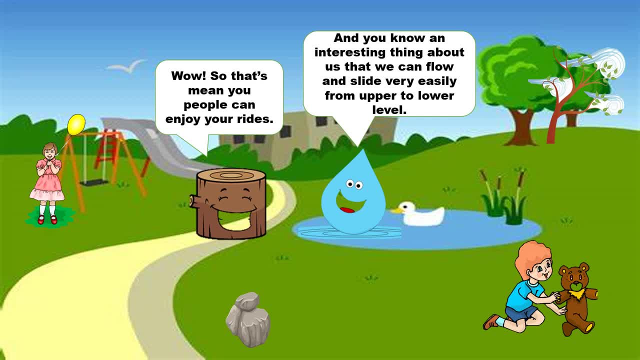 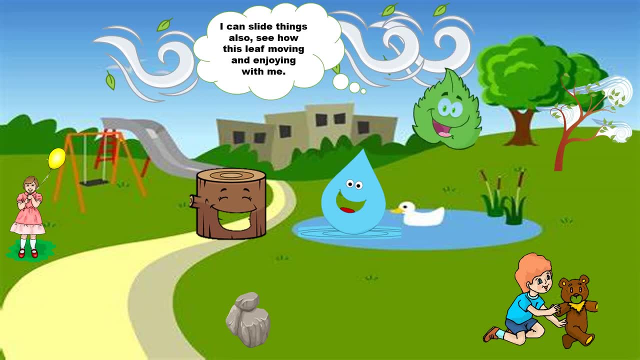 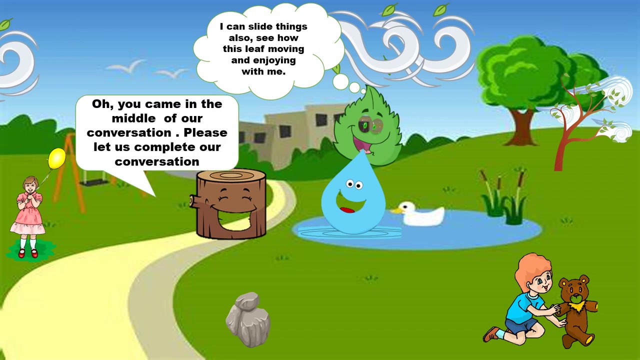 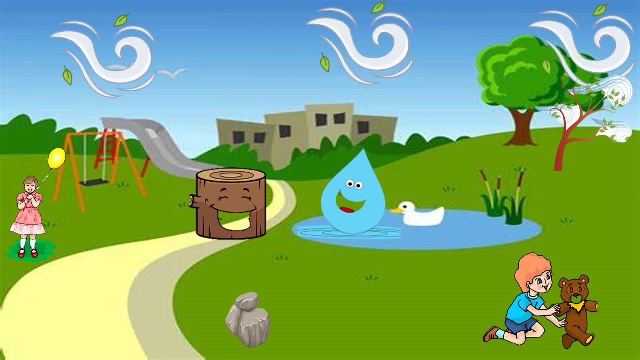 Wow, So that means you people can enjoy your rides. I can slide things also See how this leaf is moving and enjoying with me. Oh, you came in the middle of our conversation. Please let us complete our conversation. Yes, Liquid, What about your family members?